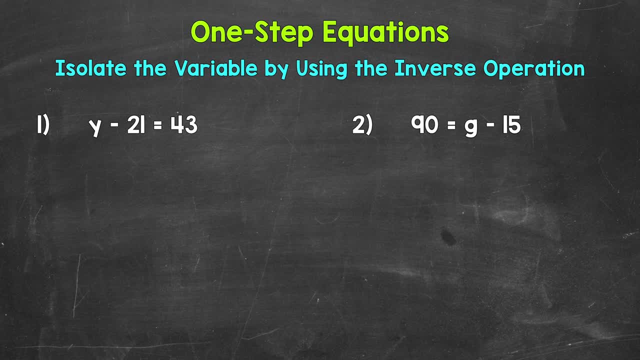 So the opposite operation, The opposite of subtraction, is addition. So let's add 21 to the left side of the equation. Now, whatever we do to one side of the equation, we must do to the other in order to keep it balanced and equal. 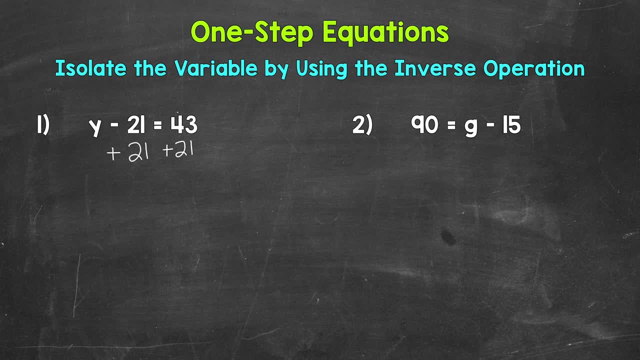 So we need to add 21 to the right side as well. Now let's take a look at the left side of the equation. We are subtracting 21 and adding 21.. So these 21s cancel out. They equal zero. 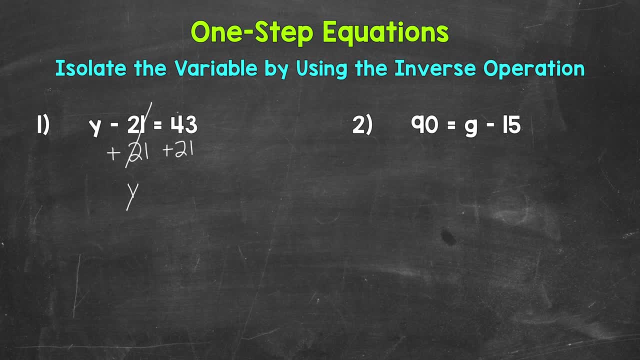 So our variable y is now isolated. It's by itself. So y equals, And then on the right side of the equation 43 plus 21.. So y equals, And then on the right side of the equation 43 plus 21.. 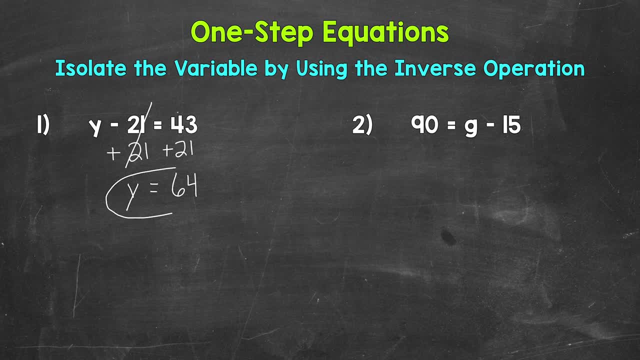 So y equals, So y equals, So y equals 64.. So y equals 64. That's our solution. Now we can always check a solution by plugging it into the original equation. So let's plug 64 in for y and see if this works. 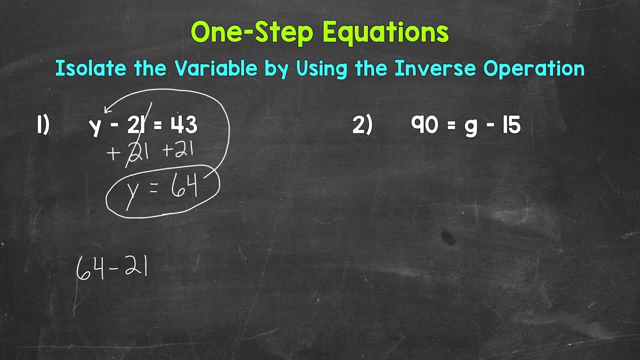 64 minus 21 equals 43.. 64 minus 21 does equal 43. So we have the correct solution: y equals 64.. Let's move on to number 2, where we have 90 equals g minus 15.. 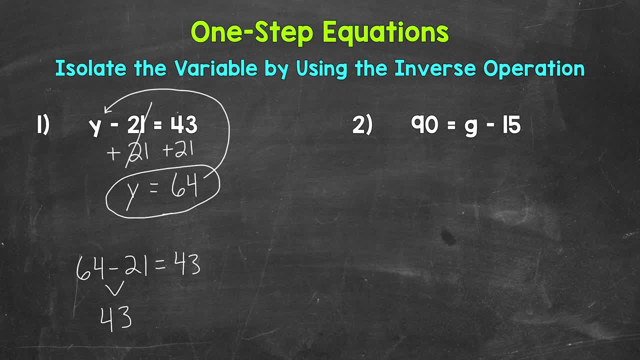 We need to isolate that variable of g. 15 is being subtracted from g, So we need to undo that subtraction by using the inverse operation. The inverse of subtraction is addition, So let's add 15 to the The right side of the equation. 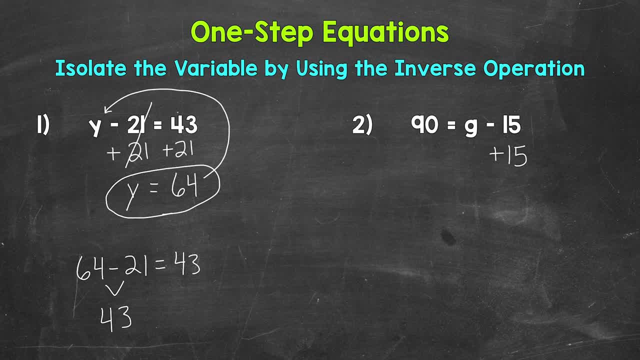 Now, whatever we do to one side of the equation, we must do to the other. So let's add 15 to this side as well. Now, on the right side of the equation, we are subtracting 15 and adding 15.. 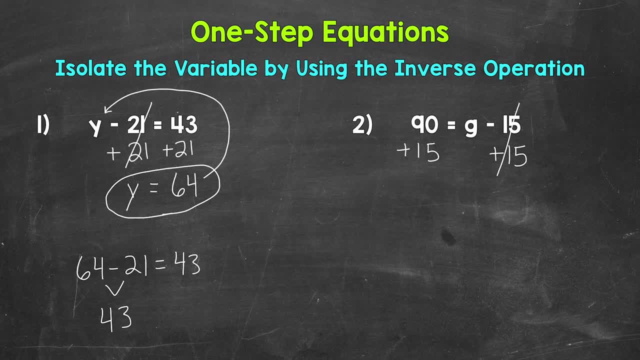 So these 15s cancel out. They equal 0.. So g is now isolated. It's by itself g equals, And then, on the left side of the equation, 90.. 90 plus 15 equals 105..